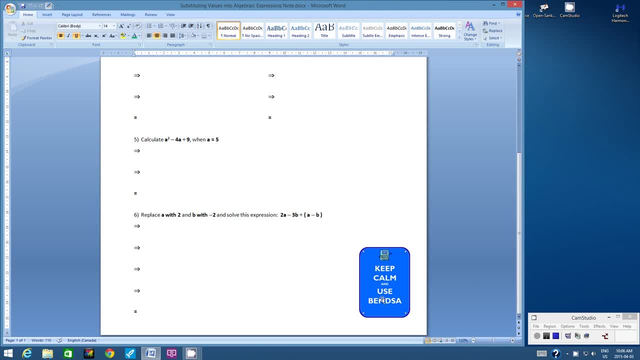 questions that you have to follow the rules of BEMSA. You must use BEMSA when you are calculating the answer. Brackets, exponents, multiplication or division in whatever order they occur, and then, lastly, subtraction or addition in whatever order they occur. Okay, so, like I said, you've done this. 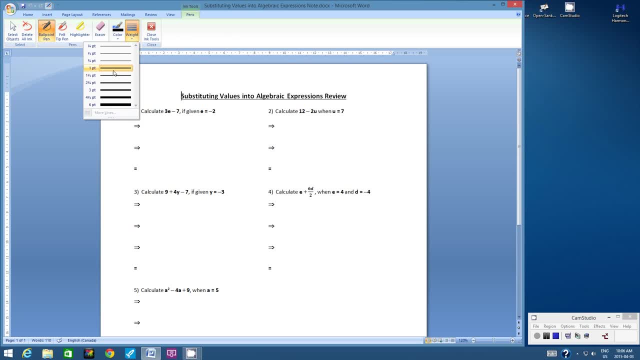 type of question before. so let's see what you remember. Okay, question number one: Calculate three questions in a row: One, two, three, four, five, six, seven, eight, nine, ten, Three e minus seven if given, the value of e equals minus two. So the reason why these questions are: 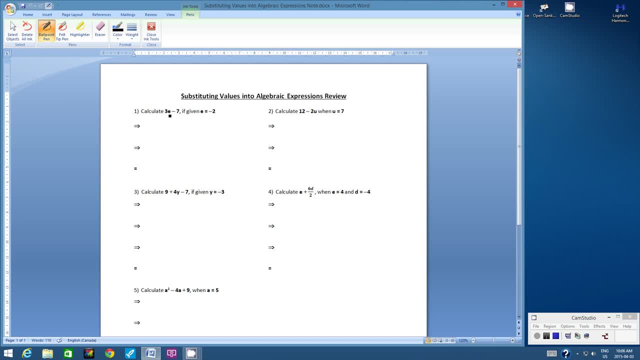 called substitution questions is, whenever you see a variable- okay, that's a letter- that variable is represented by a number, which we don't always know. In this case, we know that whatever you see e, it is represented by negative two. Okay, so three e. What you have to remember about three e is: 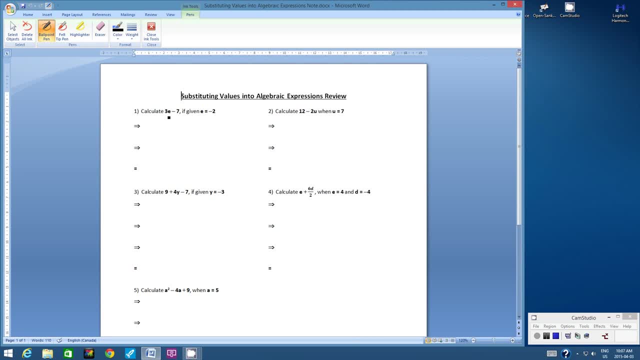 there is a hidden operation Between three and the e. Do you remember what it is? It's multiplication. Okay, so let's copy this question. So we have three and then e. What is the value of e? It is negative. two, Okay, and then we're. 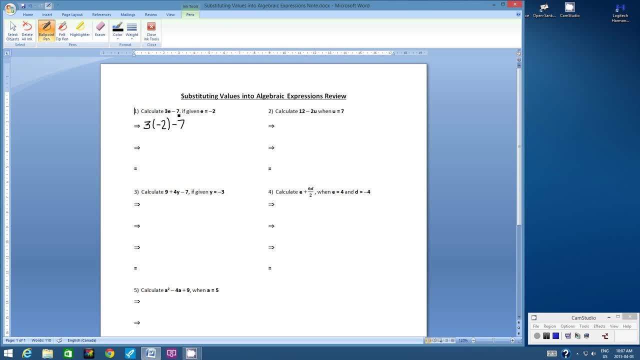 left with minus seven. The rest is the same because there's no other variables. Okay, so we have a negative seven, or we can do three times negative two. Well, if we follow the rules of BEMSA, we have to do multiplication. So, even though this is a bracket, it's a bracket around an integer, which isn't really. 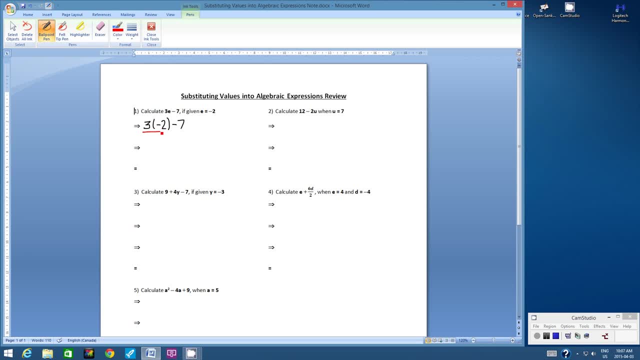 a bracket. So let's underline this part of the question, because we're doing the multiplication first. So what is three times negative two? Well, three times negative two is negative six, Okay, positive times. a negative equals a negative. All right, in the next line. here see how I've drawn an arrow to show that we're going to go to the next line. 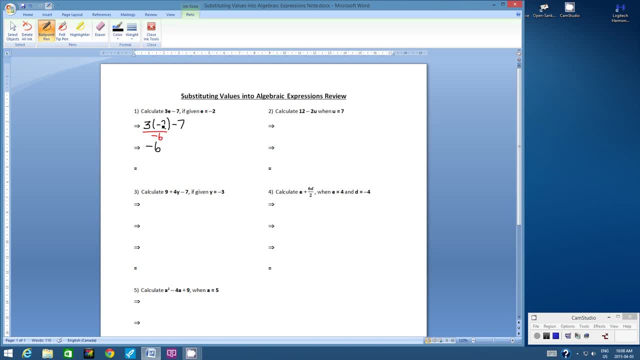 We copy negative six. That takes care of this part of the problem. And then we have negative seven. Well, using our integers of subtraction rules, negative six subtract seven is negative thirteen. Okay, All right, let's go to example two. 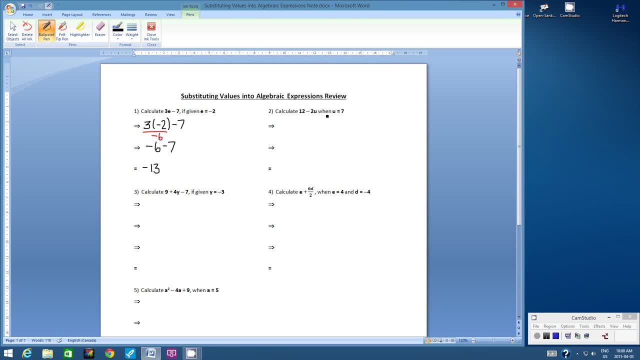 Calculate twelve minus two u when u equals seven. Okay, so let's copy the question. So twelve is unchanged Subtract two, and then we have u Remember two. u means two times u and u has a value of seven. Okay, so let's look at this. 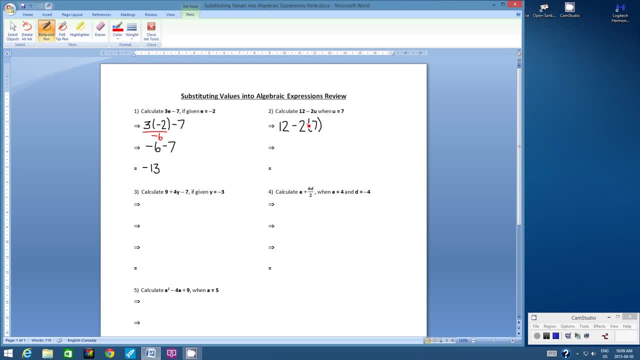 question. now We have a subtraction and we have a multiplication. Remember, this is multiplication. So, following the rules of BEMSA, we have to do multiplication first. So what is two times seven? Well, two times seven is fourteen. Okay, So let's copy down what we have left. We have twelve, which was untouched Subtract. 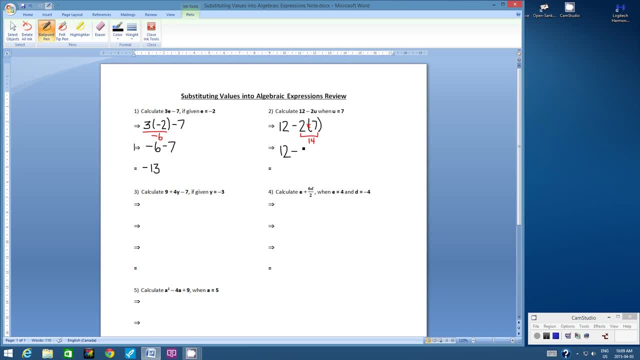 remember this is a subtraction sign, Subtract fourteen, Twelve, subtract fourteen Twelve, subtract fourteen is Negative two. Okay, All right, let's go on to example 3.. Calculate 9 plus 4y minus 7 if given the value y equals negative 3.. Okay, so we have a little bit longer question here, and maybe that's why. 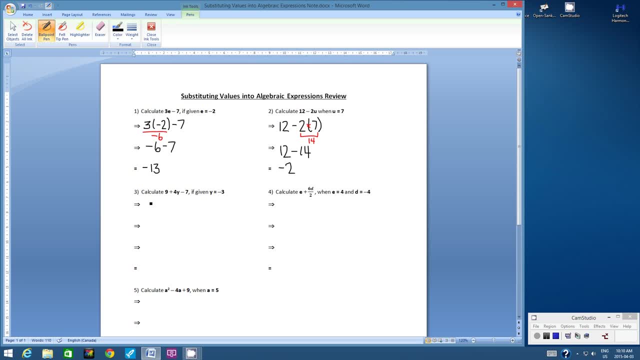 there are more than there's four lines to this solution, So let's copy down the question: 9 plus 4y. 4y means 4 times y, so we'll put a bracket here: negative 3, subtract 7.. Okay, so let's look. 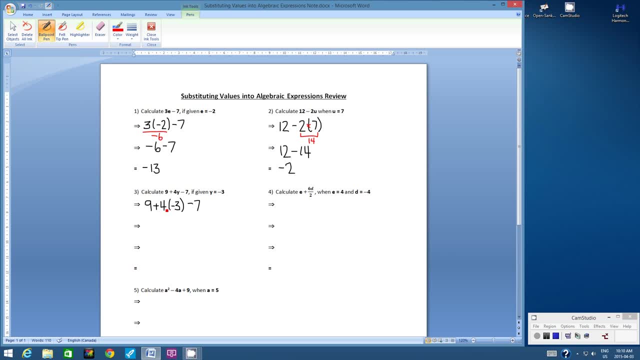 at this question. We have an addition, we have a multiplication and then we have a subtraction. Well, following the rules of BEMSA, we have to do the multiplication first. So what's 4 times negative 3? 4 times? 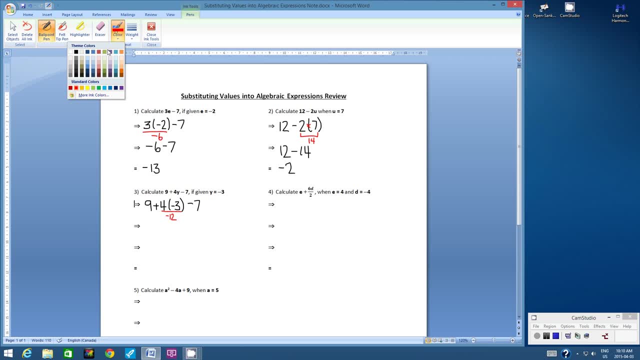 Negative 3 is Negative 12.. So let's copy what we know. after one step, We have 9 plus negative, 12 minus 7.. Okay, so let's look at the operations that remain. We have addition and we have 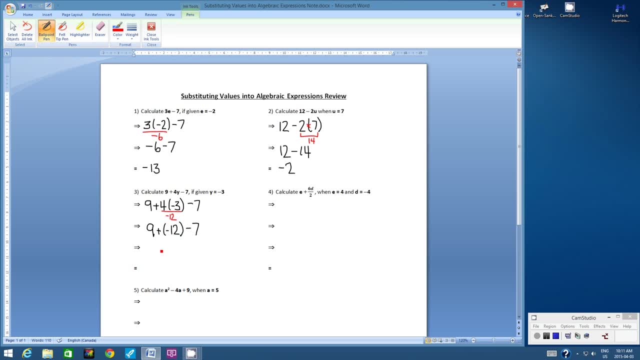 subtraction. So, following the rules of BEMSA, we do addition or subtraction in the order they occur. So in this case, addition was first 9 plus negative 12 is negative 3.. Okay, so what's left here? We have negative 3, subtract 7.. Negative 3, subtract 7 is negative 10.. So a lot of students. 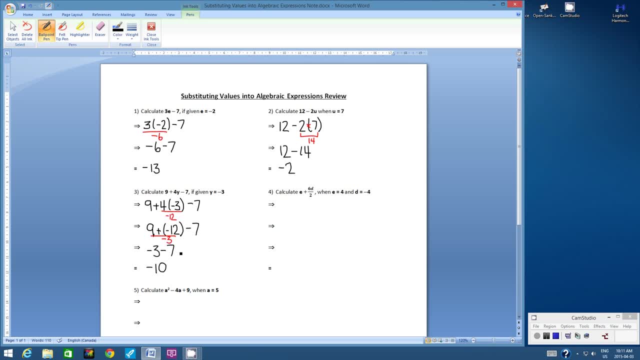 will be asking this: How do you know how many steps there are in the argument? 4 times 7 is the number of steps you have to take in order to know the number of steps. Remember, if you draw 4 times, it's going to look like this, Which means that you have to figure. 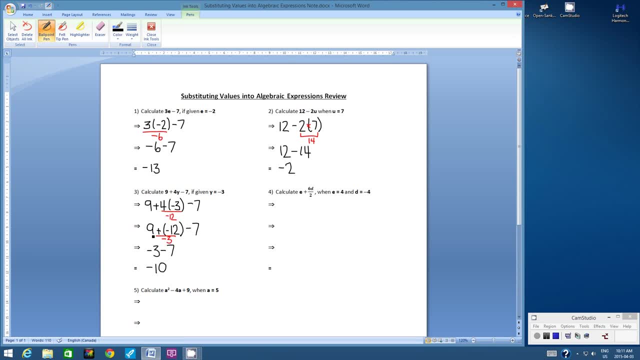 the number of steps the proper way. Number one of paths should be developed in order, Fort Meuse, the same way you did in F Superior Oldspice, New YaleessaATE. You had this answer here. You could have added 7 steps and given 9 steps. it would appear that the 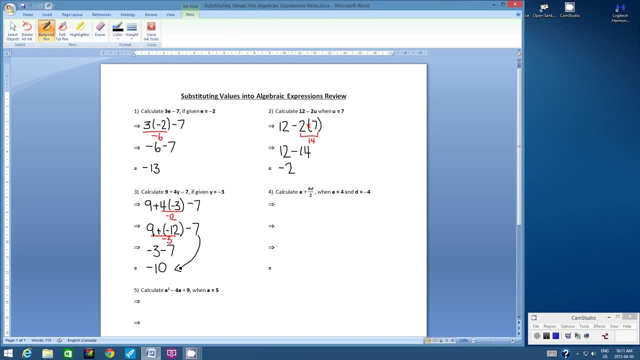 same number of steps can be combined because you had 9 steps. All right, let's look at the chess game We have: draw, prevent, subtract. The game says it looks like 4 times negative 12 minus 7, which means it is negative 9 plus negative 12 plus 7 minus 7 minus 7, so 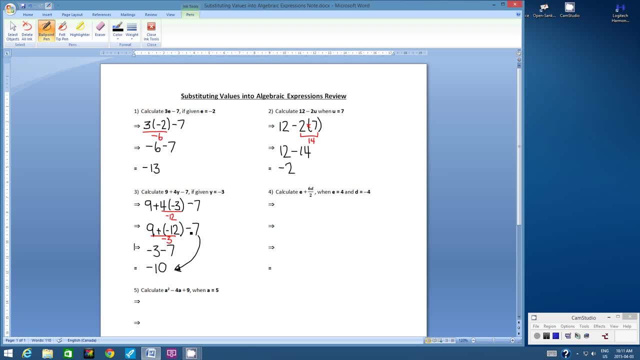 this comes in stream 9.. and the addition and the subtraction in the same line. You have to show me that you understand. you're separating the steps of BEMSA. Okay, All right, let's go on to the next one. We have something exciting here. 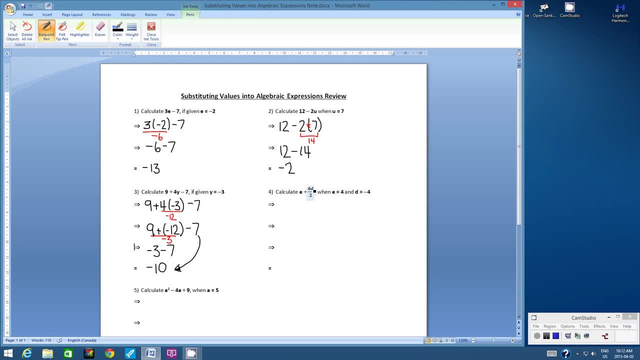 Calculate e plus 6d divided by 2, when e equals 4 and d equals negative 4.. So the exciting part about this question is we have two different variables and we have division. Okay, so let's see what this looks like. 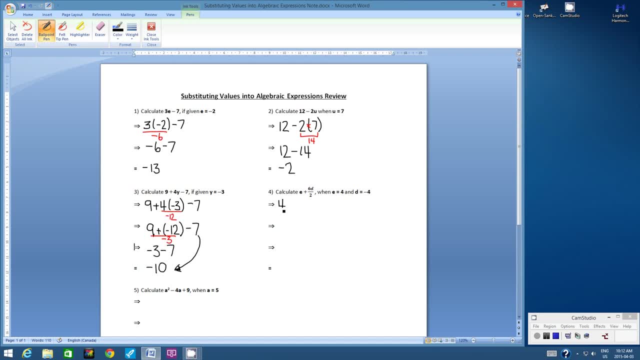 So the value of e is 4.. So let's substitute that 4 plus and we have 6d. So that means 6 times. and what's the value of d Negative 4 divided by 2.. Okay, so what steps should we concentrate on? first, 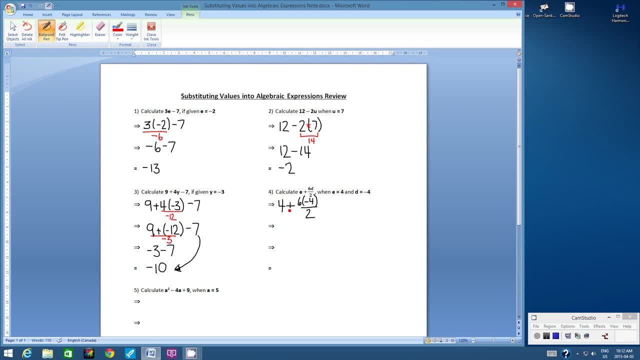 Well, we have a lot of choices. We have a division, We have addition, which we know we're not going to concentrate on. first We have division with this fraction And then we have multiplication. So let's do the multiplication first and calculate the numerator. 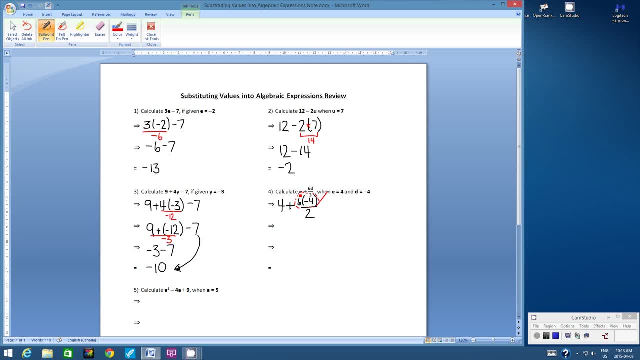 So I'm just going to draw a little dotted circle around this, Okay. So what is 6 times negative 4?? Well, 6 times 4 is 24.. And a positive times a negative is a negative. Okay, so that's step 1.. 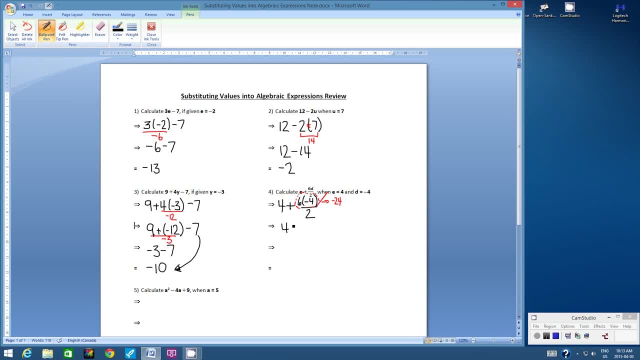 So let's copy what we know. So we have 4 that we didn't do anything to it. Plus we didn't do anything to that, We have negative 24 divided by 2.. Now, remember, fraction means division. Now, if you want to put a bracket around this, that's fine. 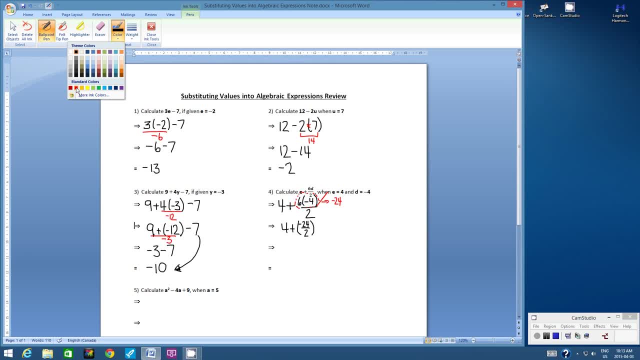 Just so that you can isolate it. That's cool, Okay, so let's do the division. Remember: this means negative 24 divided by positive, 2.. Negative divided by a positive is going to be a negative. 24 divided by 2 is 12.. 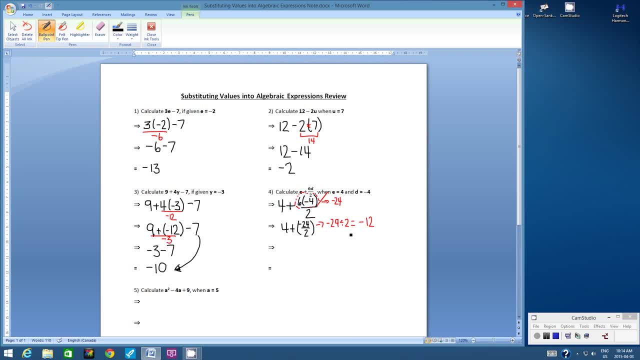 Okay, So you see how I'm showing all my work on each step. Then we have 4 plus and then we're left with negative 12.. Okay, All right, 4 plus negative 12.. What's 4 plus negative 12?? 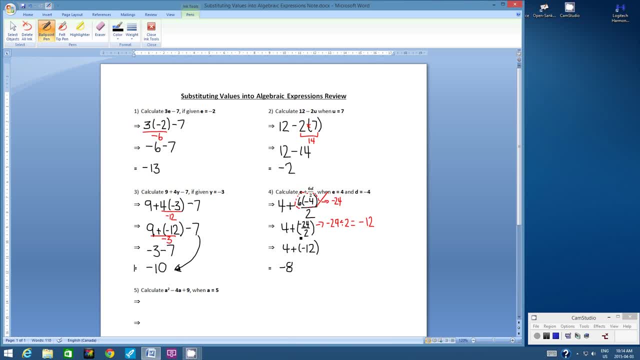 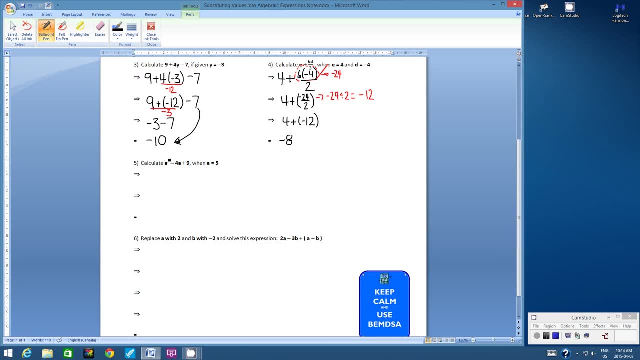 Negative 8.. Okay, So let's move on to example 5.. a squared minus 4a plus 9 when a equals 5.. So what's different about this question? We have an exponent Excellent, All right, so let's do our substitution line. 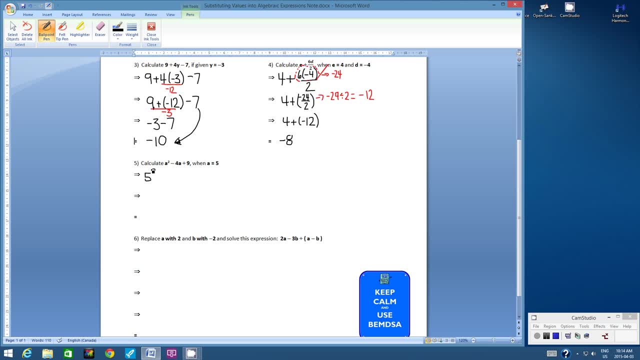 a is 5.. 5 squared 5.. Minus 4a: 4a means 4 times 5, so 4, bracket 5.. Now remember: when we put a number next to a bracket, it means multiplication. 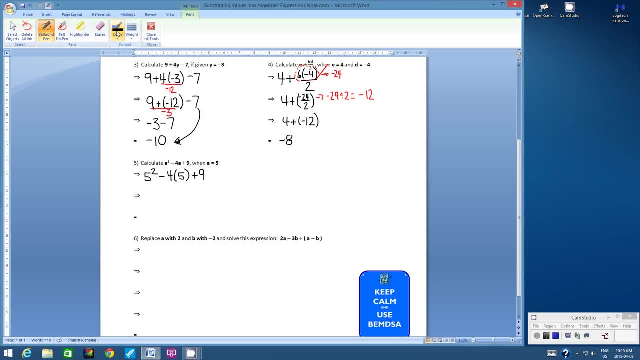 Plus 9, okay. So, following the rules of BEMSA, what do we do first? Well, we do exponents. Now, remember, this is technically not a bracket in the BEMSA world. okay, So 5 squared. 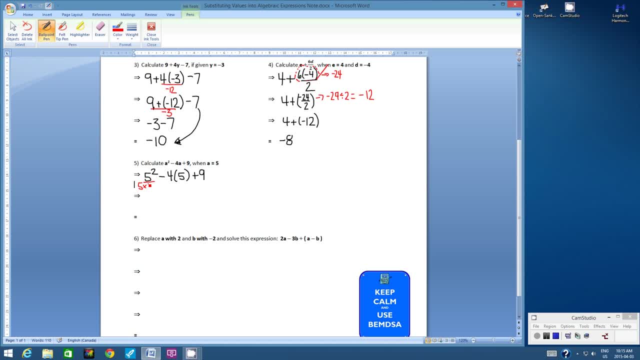 Now remember: 5 squared is not 5 times 2.. 5 squared is 5 times 5,, which is 25.. Now, when you're solving these questions, you don't have to write 5 times 5.. I just want you to write it in this note. 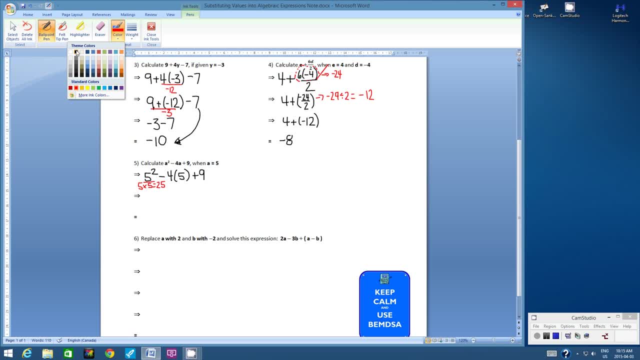 so that you remember what exponents mean. That is the most common error when working with exponents. Okay, so we solve the 5 squared. We have 25 minus 4 times 5, plus 5.. Plus 9, okay. 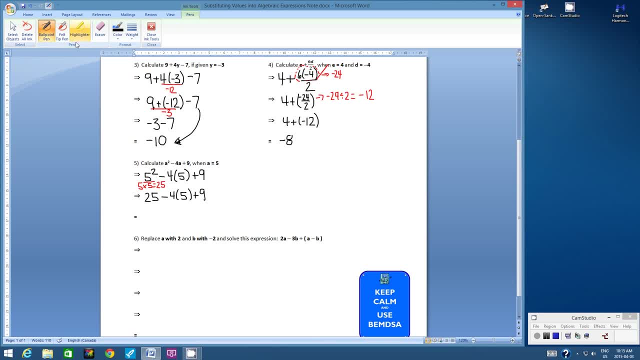 Now, what we could have done here is we could have done this step in the same line, the multiplication. But what we'll do is we'll add another line here. So let's do this: multiplication 4 times 5 is 20, okay. 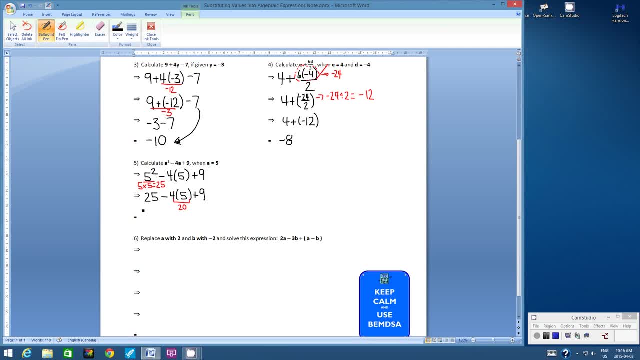 4 times 5 is 20.. So we have 25 subtract 20. So we have 25 plus 9.. So whenever we're left with only subtraction and addition, you can just go left to right and do all the steps at once, okay. 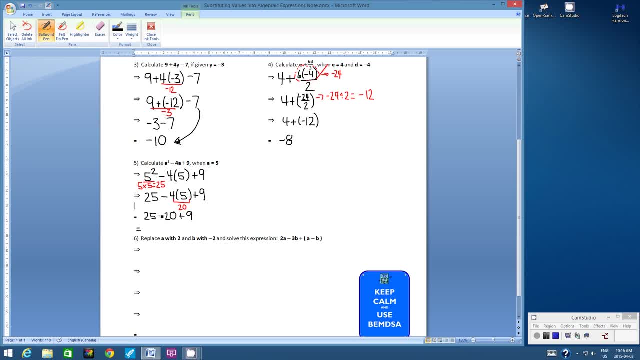 So I'm going to add a line here. So we have 25 subtract 20 is 5.. 5 plus 9 is 14, okay, All right. So let's look at example 6.. Replace a with 2 and b with negative 2 and solve this expression. 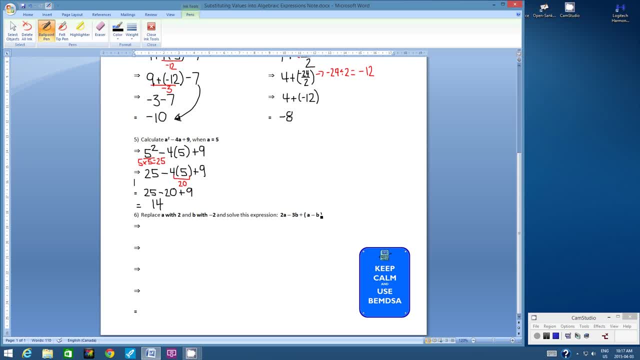 2a minus 3b, plus bracket a minus b, So we get a bracket in this question. Awesome, Okay. so let's start substituting So 2a, which is 2 times 2.. a is, remember, positive 2.. 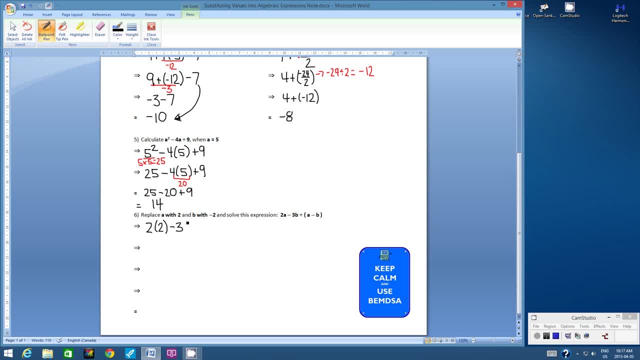 Subtract 3b 3 times And b is negative 2. Plus a, which is 2. Subtract b, which is negative 2.. Okay, So you'll never be able to get these questions correct if you can't substitute correctly. 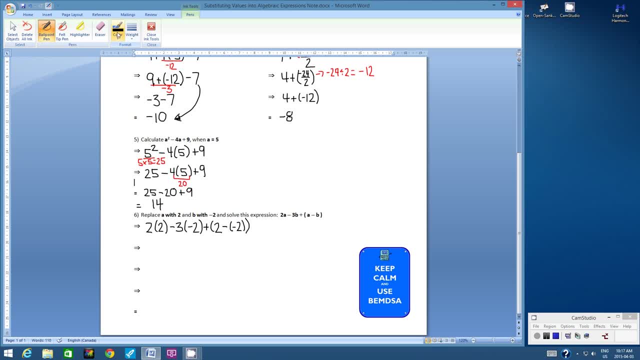 Okay. So we've got a lot going on here. So because we have a true bracket, according to the rules of BEMSA we have to solve the bracket first. So what is 2 subtract negative 2?? Well, this is actually 2 plus positive 2, isn't it? 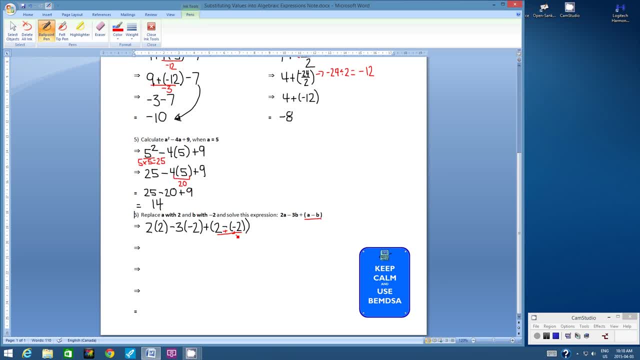 And that equals positive 4,. okay, All right, So let's copy down. Let's copy down what we know. This part was unchanged: 2 times 2.. Subtract: 3 times negative 2. Plus, remember, this was a plus. 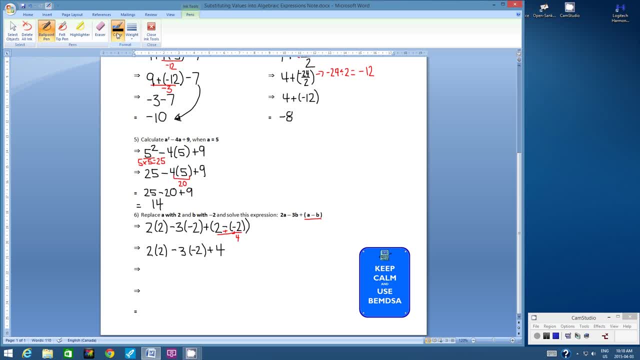 And we have positive 4 here. Okay, So let's see what's going on now. We have multiplication, We have subtraction, We have multiplication And we have an addition. So, according to the rules of BEMSA, we have to do the multiplication first. 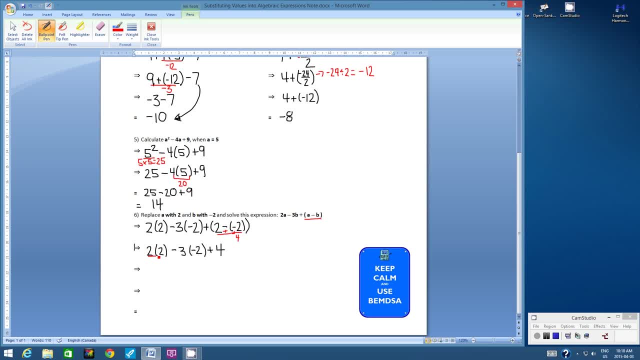 Now there are two multiplications, So why don't we do both multiplications at the same time? 2 times 2 is 4.. 3 times negative: 2.. 3 times negative: 2 is negative, 6.. All right, 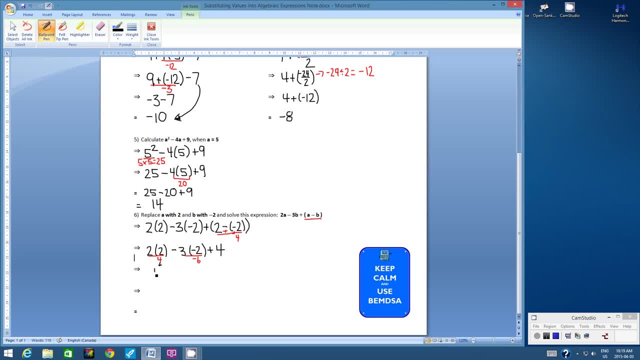 So let's copy down what we know. This is 4. Subtract. This is subtract Negative: 6. Plus 4.. Okay Now, because we're left with only subtraction and addition left, we can just go left to right if you want. 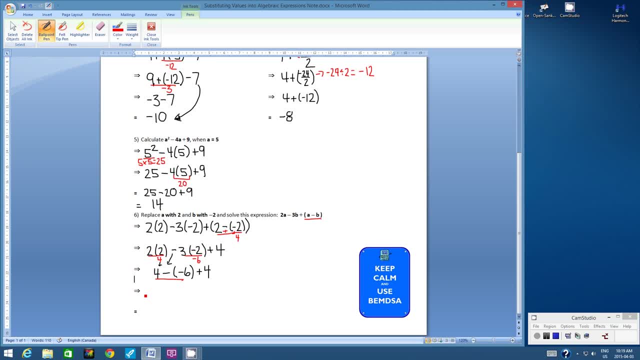 Or we can just do them one step at a time. So because I've got two lines left, I'm going to do them one step at a time, But you can do both of these steps at the same time. So 4 subtract negative 6..